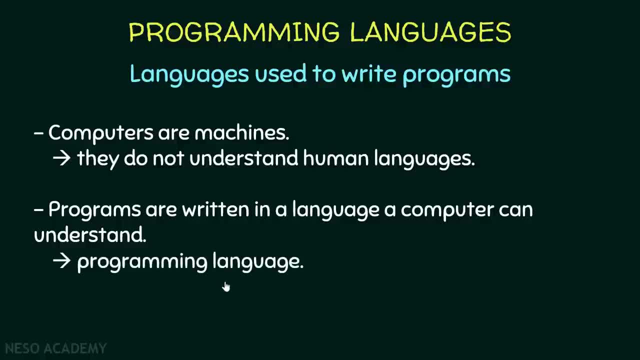 That a computer can understand, which is a programming language. So to be able to interact with a computer, we should write programs using a language that a computer can understand, which is a programming language. Now let's see. what do we mean by machine language? 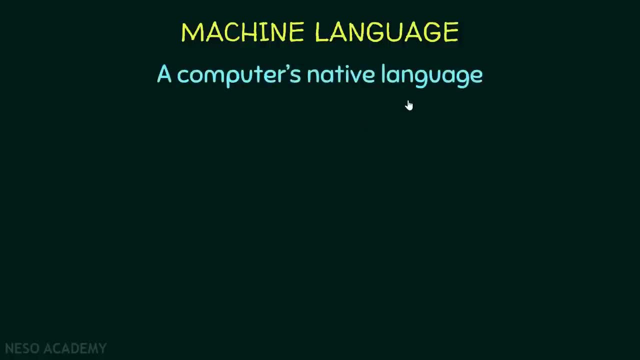 This is the computer's native language, So it is the main language of the computer. This language uses zeros and ones, So the digit zero and the digit one, And this is why it is called a computer And this is why it is called the binary language. 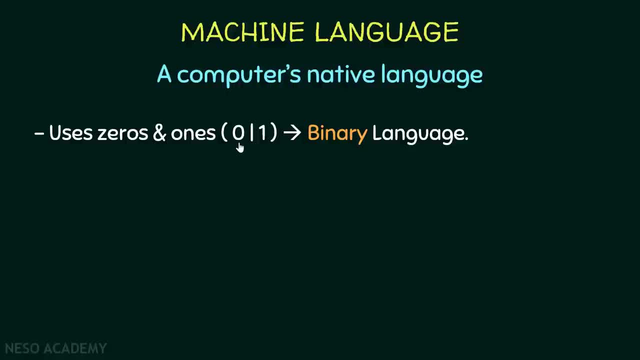 Binary means two things, So, as you can see, we are using two digits, The zero and the one. So, for example, if we want to add two numbers, two and three- and get the result, we would write something like this: 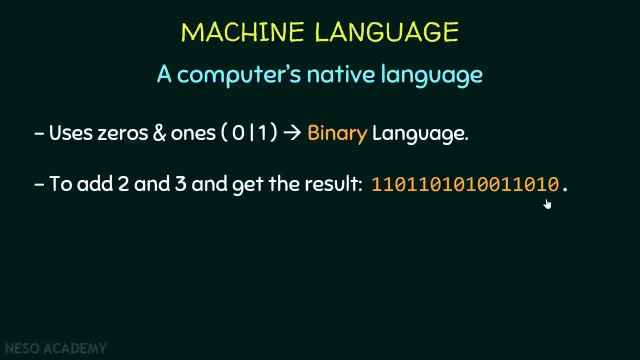 This is an instruction written using the machine language. It is a group of ones and zeros, as you can see, And this is only one instruction: just to get the sum of two and three and get the answer, which is four. And this is only one instruction: just to get the sum of two and three and get the answer, which is four. 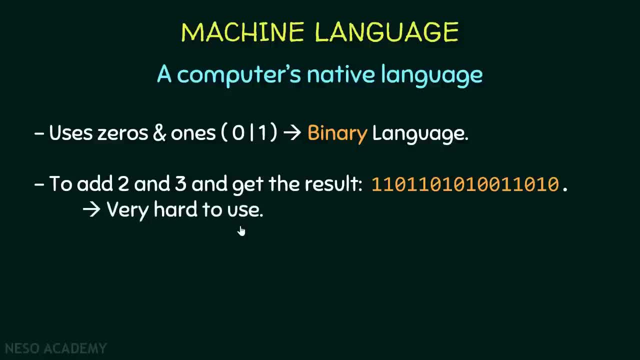 So, as you can see, this is very hard to use. Moreover, machine language is machine dependent, So it differs among different types of machines. So this code over here might work on a certain machine and it might not work on another machine. So this is what we mean by machine dependent. 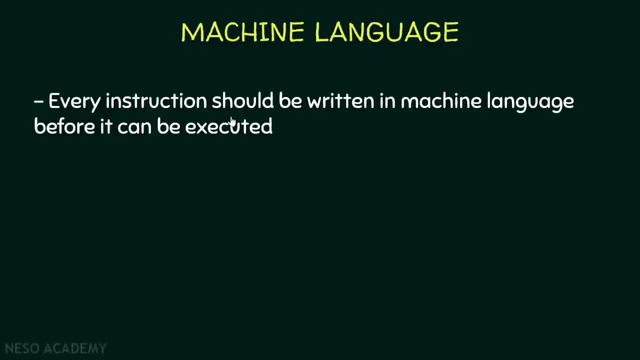 Now let me tell you this: Every instruction should be written in machine language before it can be executed. So later on we're going to write programs using Java, So the instructions will be written using the Java programming language. So all of those instructions must be translated to machine code before we can execute them. 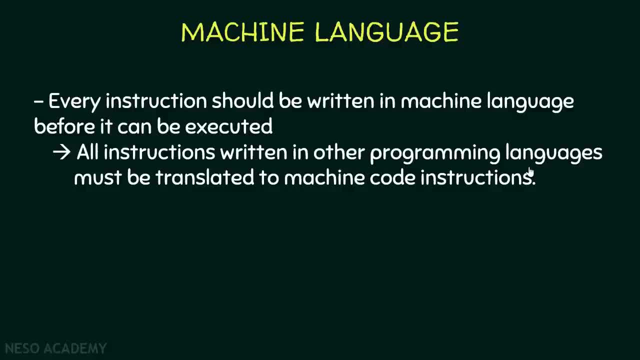 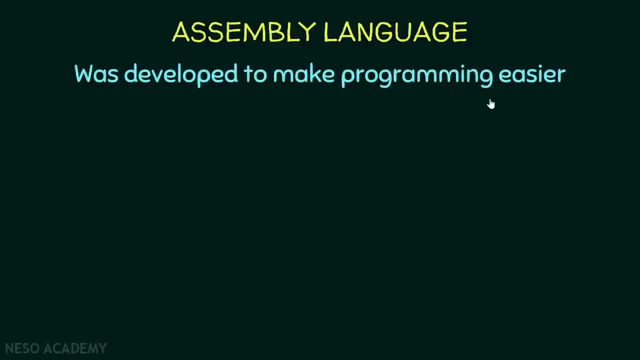 And this applies to all other programming languages. Now let's talk about the assembly language. It was developed to make programming easier. First of all, it is also machine dependent, And in the assembly language, keywords were introduced. For example, we have a keyword add and a keyword submit. 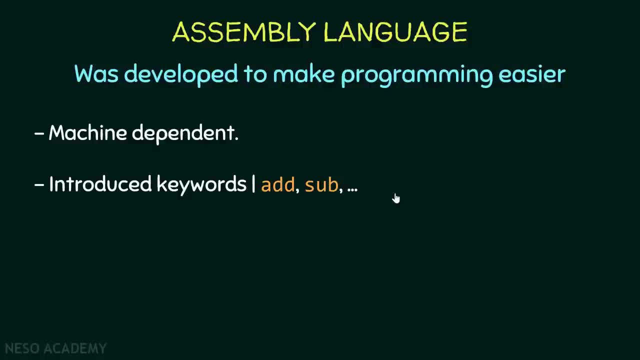 And a lot more, So programming was a little bit easier. For example, if we want to add 2 and 3 and get the result, we will write something like this: This is an assembly instruction. We are telling the computer to add the number 2 and the number 3 and to store the result somewhere called result. 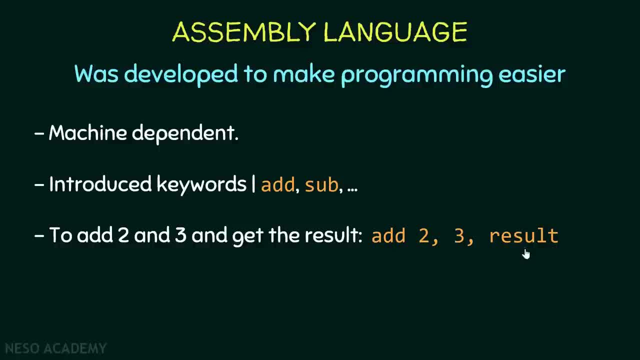 So this is an instruction written in the assembly programming language, So this cannot be executed Because, as we said, All instructions should be written in machine code before we execute them. So there is a program called assembler that translates assembly code to machine code. 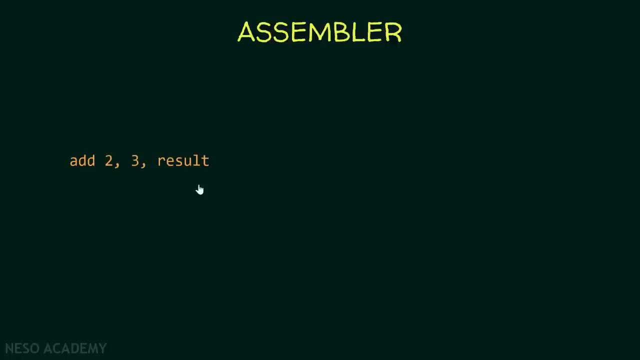 So let's talk about the assembler. Suppose that we have this assembly code over here. As we said, it cannot be executed. So this code is given to the assembler And the assembler translates this code to machine code And now this code over here can be executed. 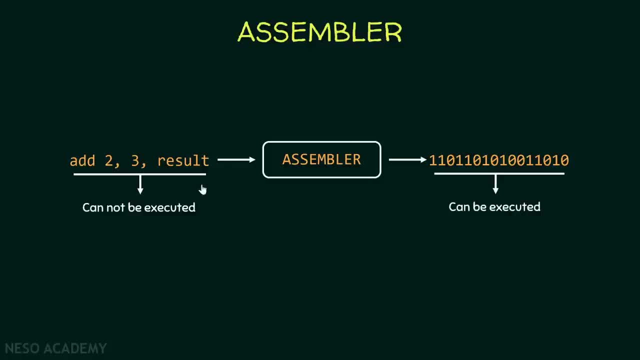 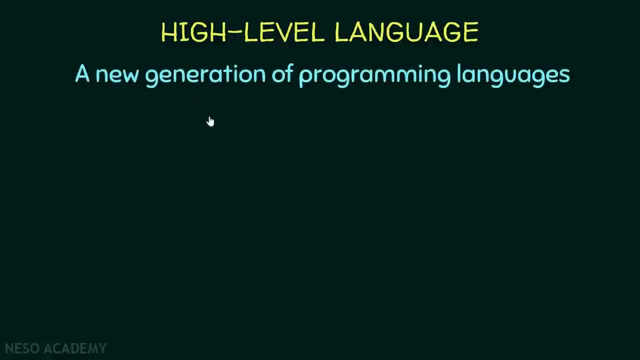 And this is how we can execute assembly code. So whenever we write a program using assembly, we will translate it to machine code using the assembler And then we will execute it. So now let's talk about high-level languages. So high-level languages are a new generation of programming languages. 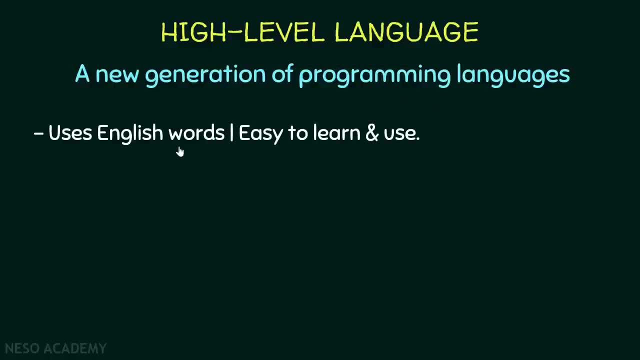 In a high-level programming language, we use English words, So this is why a high-level programming language is easy to learn and easy to use. Also, high-level languages are machine independent, So our program will run on different machines, And this is very important. 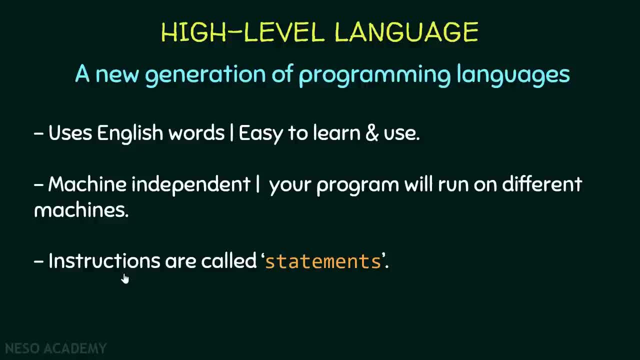 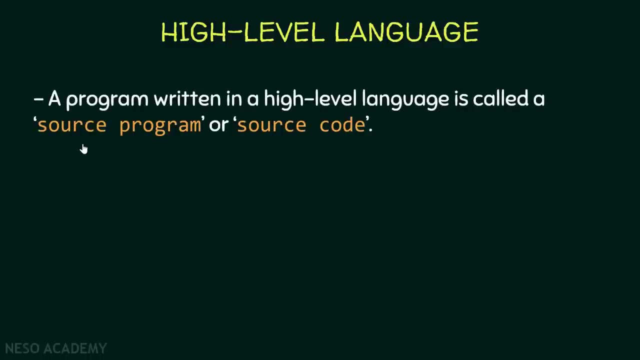 And each instruction written in a high-level programming language is called a statement. So later on, whenever we write an instruction using Java, for example, we will call it a statement, And a program written using a high-level programming language is called a source program or source code. 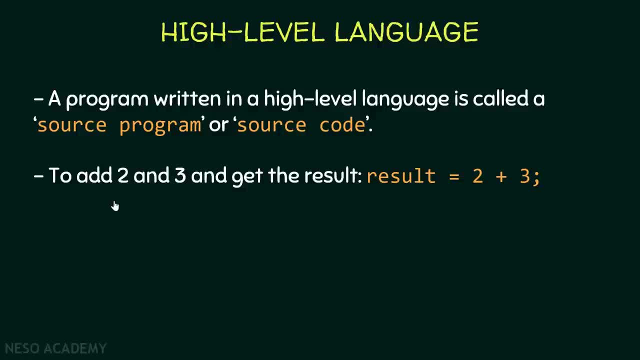 And now let's see this example. If we want to add 2 and 3 and get the result, we would do something like this in Java. This is an instruction written using a high-level programming language, So this is a statement, And this is very similar to mathematics, right? 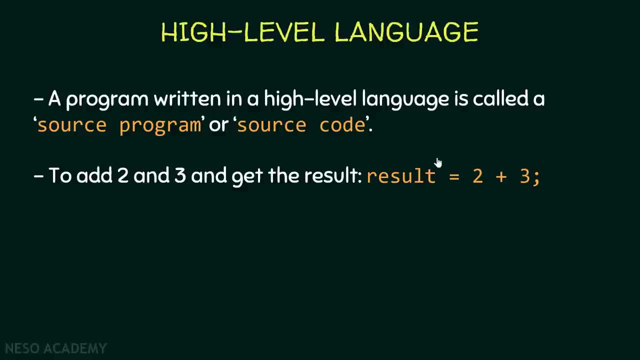 We are saying that we want to store inside result the answer of 2 plus 3.. So 2 plus 3 will be calculated, So we get 5.. And 5 will be stored in the variable result. In mathematics we have the concept of a variable right. 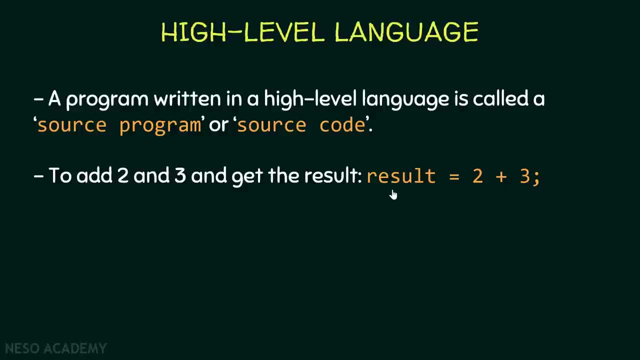 And also in programming we have variable. If you don't know what is a variable, no problem, I'm going to explain it from scratch. But for now look at this expression and see how much it is easier than assembly and machine code. 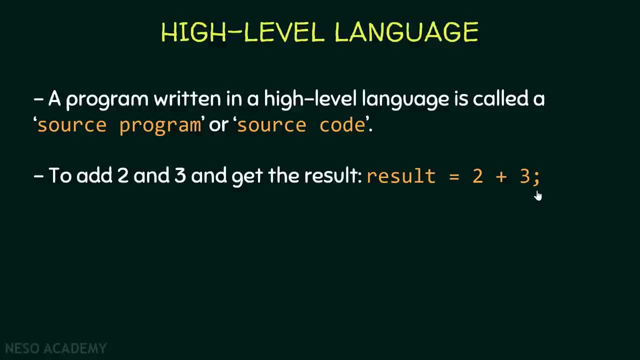 And look at this semicolon over here. Basically, every instruction or every statement should end with a semicolon, And you will see this later on. Now, just like before, this is a statement written using a high-level programming language, So it cannot be executed. 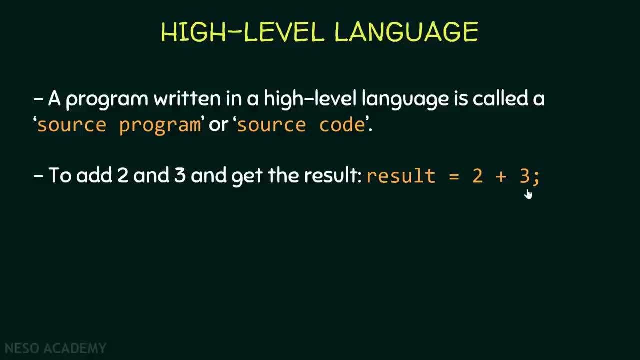 We should translate it to machine code and then we can execute it. So we can use what's called a compiler or an interpreter in order to translate a source code to machine code. And remember, source code is a program written using a high-level programming language. 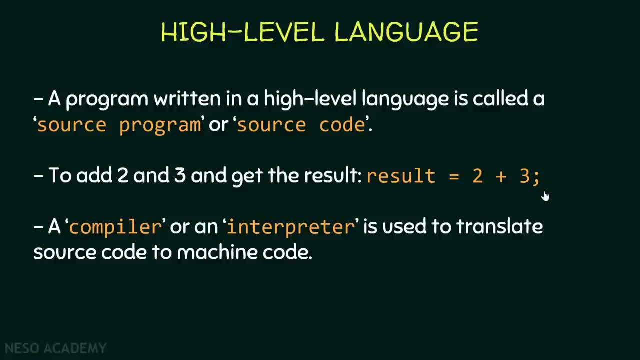 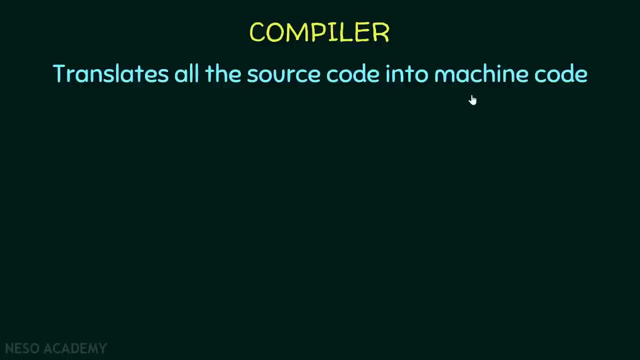 So, for example, this statement over here is a source code because it is written in a high-level language. So let's see how we can translate this statement to machine code Using a compiler. So basically, a compiler translates all the source code into machine code. 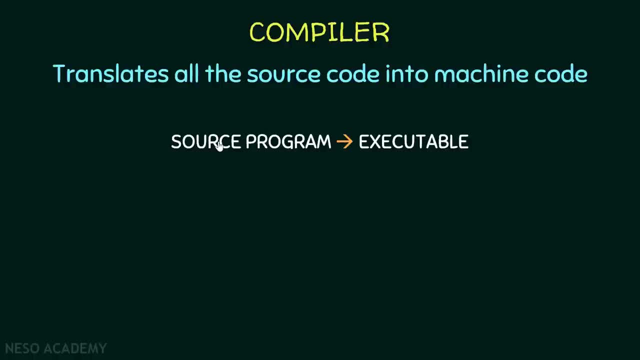 So we have a source program or a source code and we will use a compiler to get an executable. An executable is a file that can be executed by our computer. So let's have a look. We have the source code over here and we use the compiler to generate the machine code. 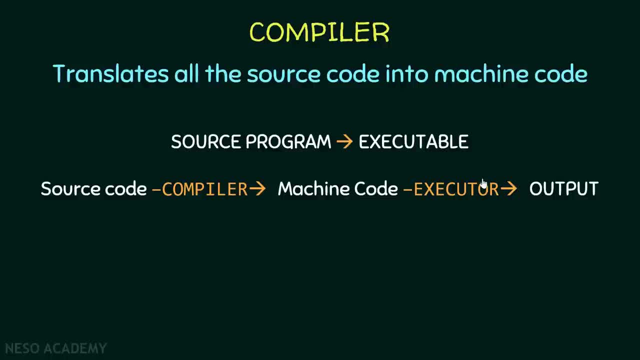 And whenever we generate the machine code, we can execute it here Using an executor, to see the output or the result. So the compiler converts all the source code or all the program to machine code And then we can execute it to see the output. 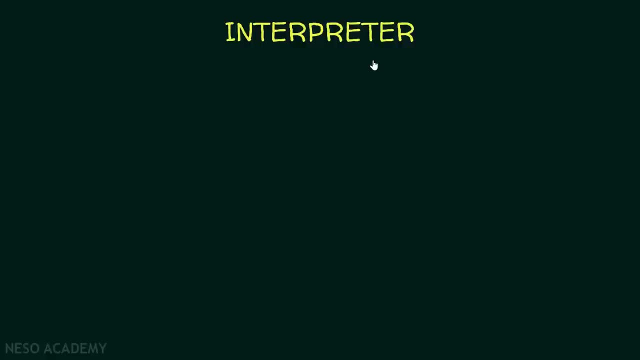 Now let's have a look at the interpreter. It works a little bit different. An interpreter translates each statement into machine code and executes it right away, So it will not translate all the program. It translates each statement at a time, So we have something like this: